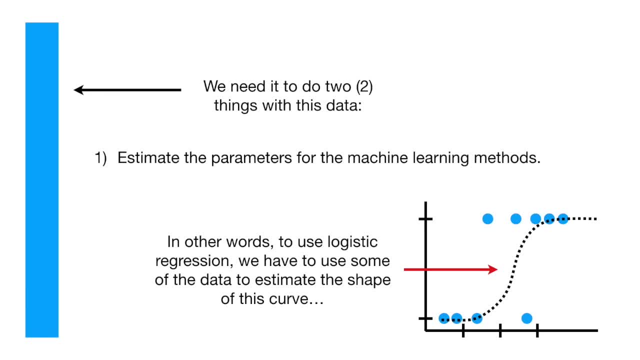 the machine learning methods, In other words, to use logistic regression. we have to use some of the data to estimate the shape of this curve. In machine learning lingo, estimating parameters is called training the algorithm. The second thing we need to do with this data. 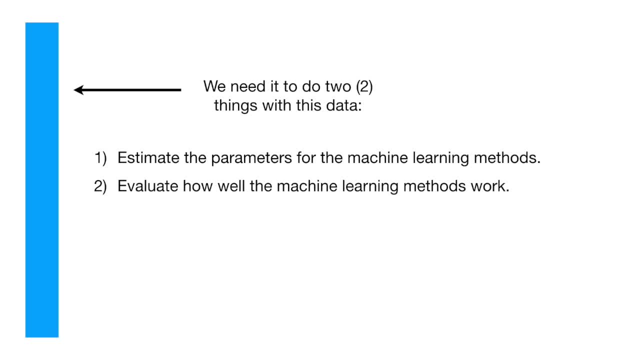 is evaluate how well the machine learning methods work. So we're going to need aі. In other words, we need to find out if this curve will do a good job categorizing new data. In machine learning lingo, evaluating a method is called testing the algorithm. 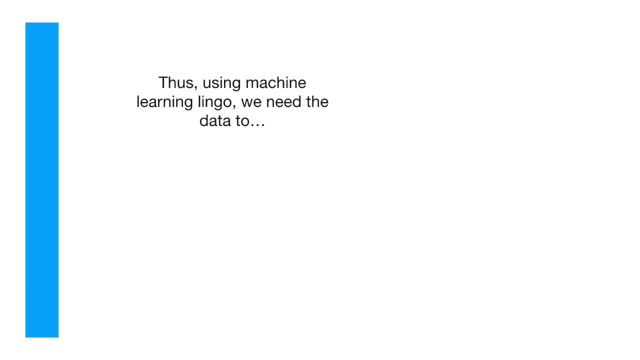 Thus using machine learning lingo. we need the data to 1. Train the machine learning methods and 2. Test the machine learning methods. A terrible approach would be to use all the data to estimate the parameters, ie to train the algorithm. 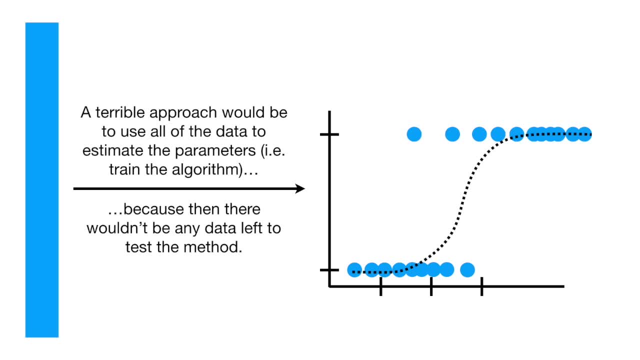 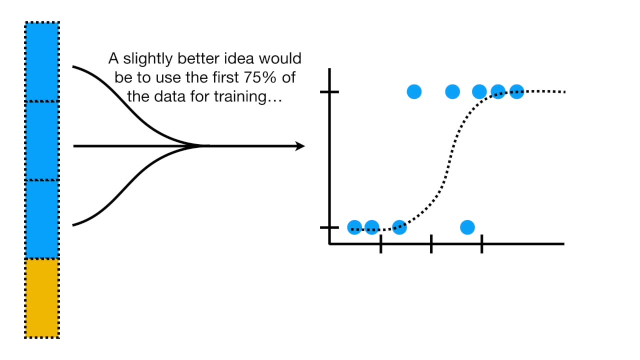 Because then we wouldn't have any data left to test the method. Reusing the same data for both training and testing is a bad idea, because we need to know how the method will work on data it wasn't trained on. A slightly better idea would be to use the 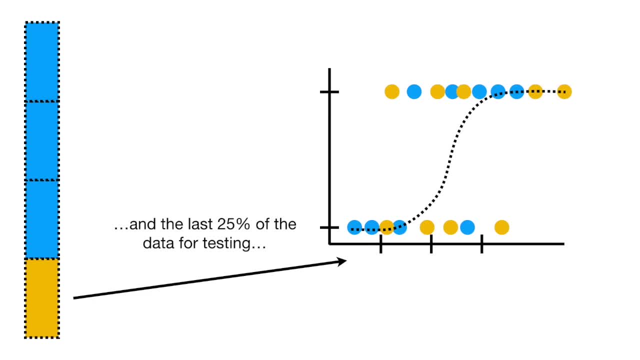 first 70% of the data to test the algorithm, Using the first 75% of the data for training and the last 25% of the data for testing. We could then compare methods by seeing how well each one categorized the test data. 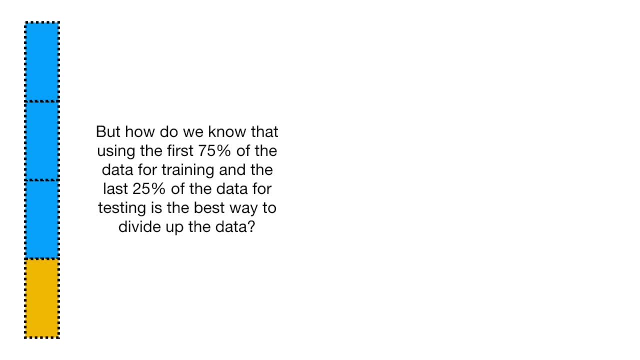 But how do we know that using the first 75% of the data for training and the last 25% of the data for testing is the best way to divide up the data? What if we use the first 25% of the data for testing? 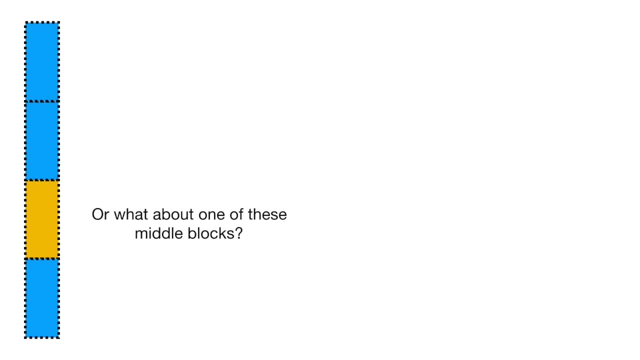 Or what about one of these middle blocks? Rather than worry too much about which block would be best for testing, cross-validation uses them all one at a time and summarizes the results at the end. For example, cross-validation would start by using the first three blocks to train the method. 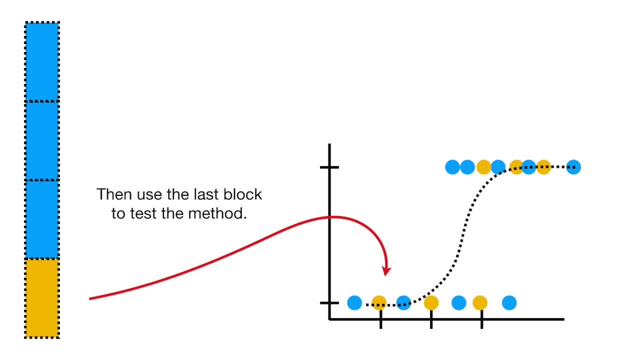 And then use the last block to test the method And then it keeps track of how well the method did with the test data. Then it uses this combination of blocks to train the method And this block is used for testing, And then it keeps track of how well the method did with the test data. 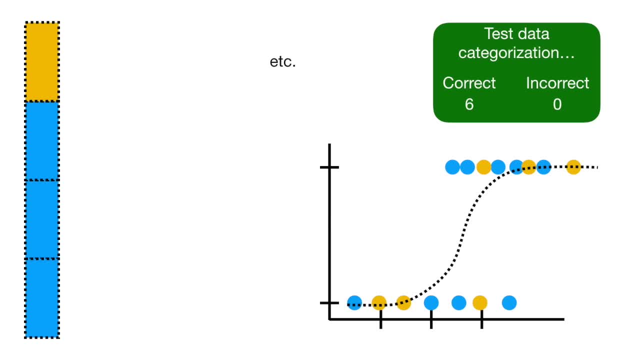 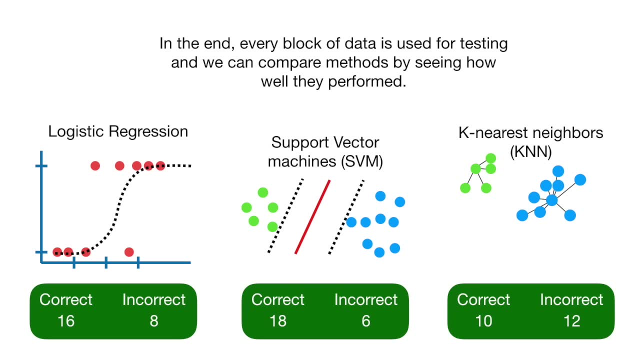 Etc, etc. etc. In the end, every block of data is used for testing and we can compare methods by seeing how well they perform. and we can compare methods by seeing how well they perform In this case, since the support vector machine did the best job classifying the test datasets. 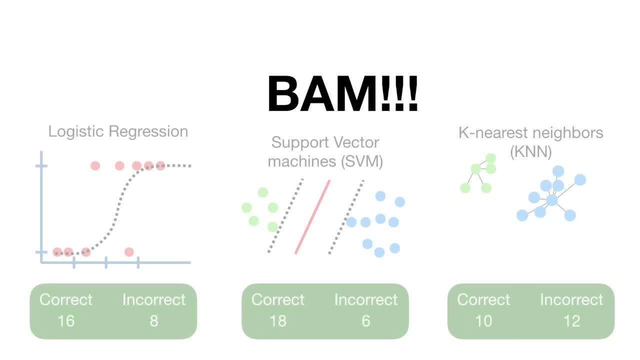 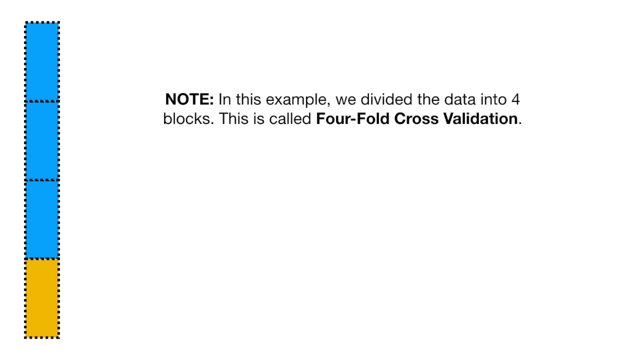 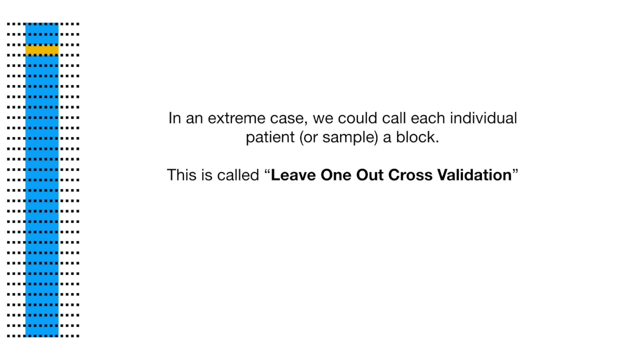 we'll use it BAM. In this example, we divided the data into four blocks. This is called four-fold cross-validation. However, the number of blocks is arbitrary. In an extreme case, we could call each individual patient or sample a block. 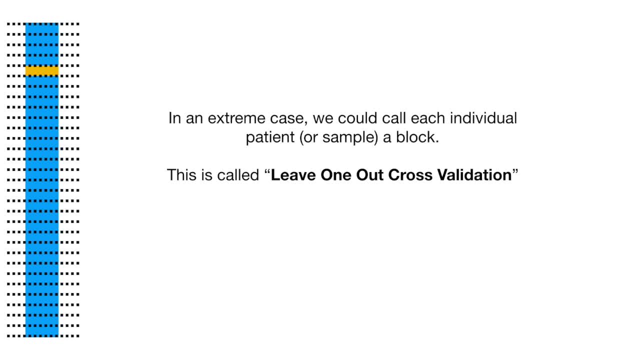 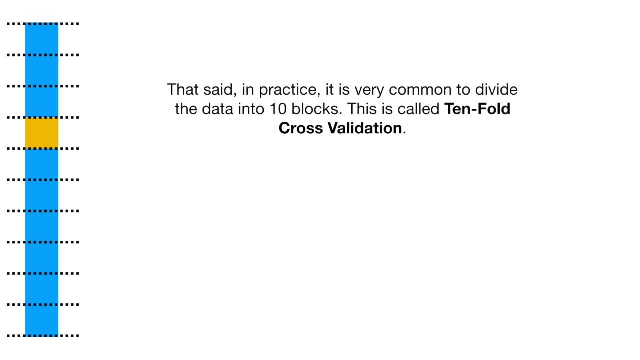 This is called leave-one-out cross-validation. Each sample is tested individually. That said, in practice it is very common to divide the data into ten blocks. This is called ten-fold cross-validation, Double BAM. One last note before we're done. 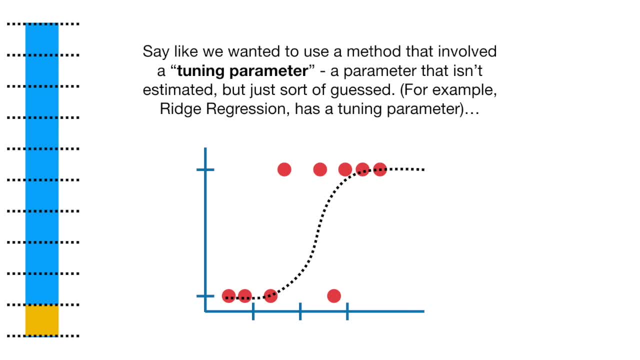 Say, like we wanted to use a method that involved a tuning parameter, a parameter that isn't estimated but is just sort of guessed. For example, ridge regression has a tuning parameter. Then we could use ten-fold cross-validation to help find the best value for that tuning parameter. 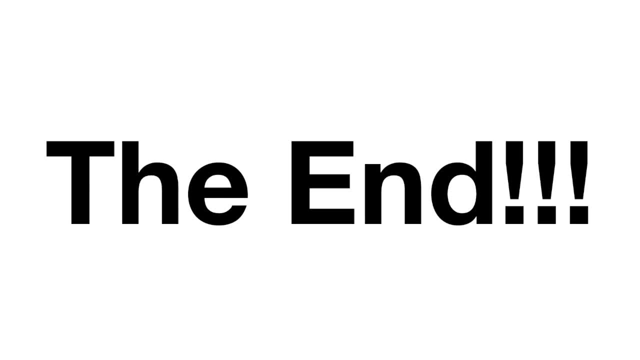 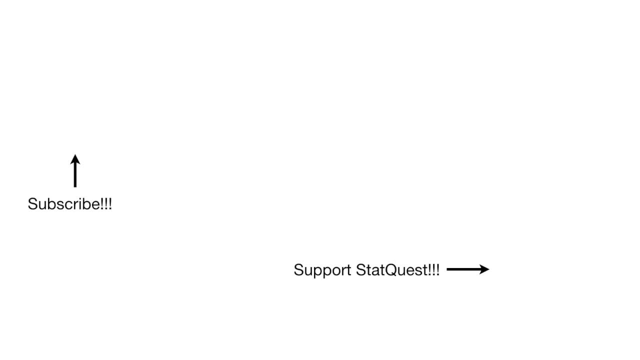 Tiny BAM Hooray, We've made it to the end of another exciting StatQuest. If you like this StatQuest and want to see more, please subscribe. And if you want to support StatQuest well, please click the Like button down below. 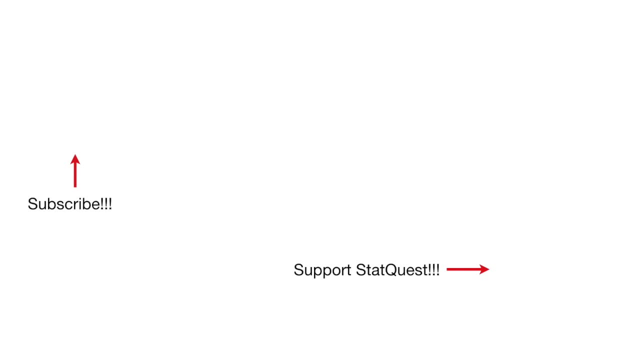 and consider buying one of my original songs. Alright, until next time. Quest on.